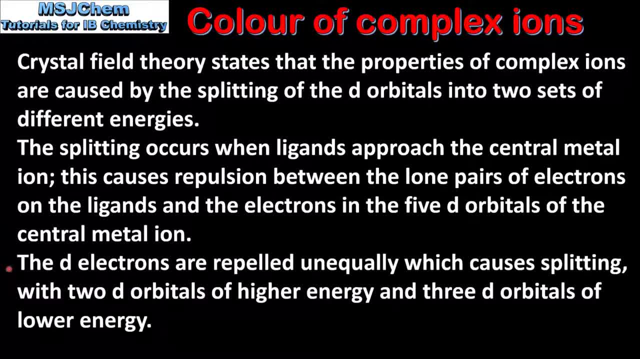 of the central metal ion, The d-electrons are repelled unequally, which causes splitting with two d-orbitals of higher energy and three d-orbitals of lower energy. Next we look at the crystal field splitting in an octahedral field of ligands. This splitting occurs when electrons in the central metal 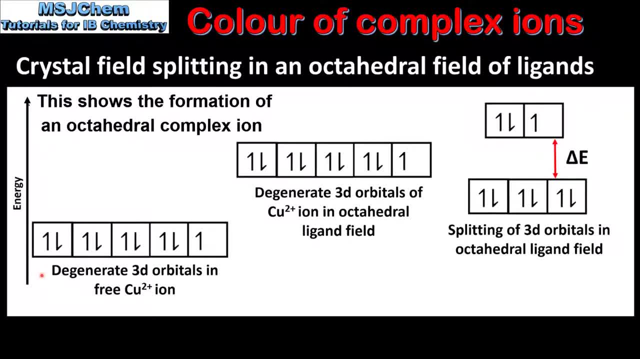 ion meet. So on the left we have the five degenerate 3d orbitals in a free copper 2 plus ion. As the ligands approach the central metal ion, the repulsion causes the five 3d orbitals to increase in energy. Because of the unequal repulsion we have splitting of the 3d orbitals. 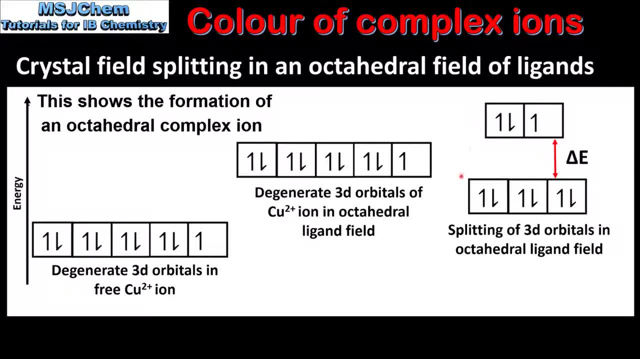 Two 3d orbitals are of higher energy and three 3d orbitals are of lower energy. So, to summarize, the splitting of the 3d orbitals occurs because of the repulsion between the lone pairs of electrons on the ligands and the electrons in the five 3d orbitals of the copper 2. 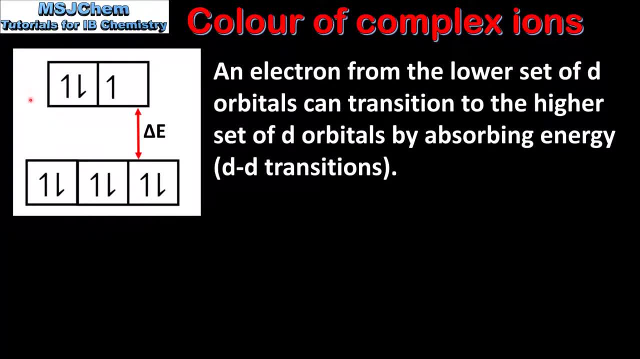 ion. So in the previous slide we saw that the five 3d orbitals split into two sets: Three orbitals of lower energy and two orbitals of higher energy. An important point to note is that transition elements have an incomplete transition element. The transition elements have an incomplete transition element. 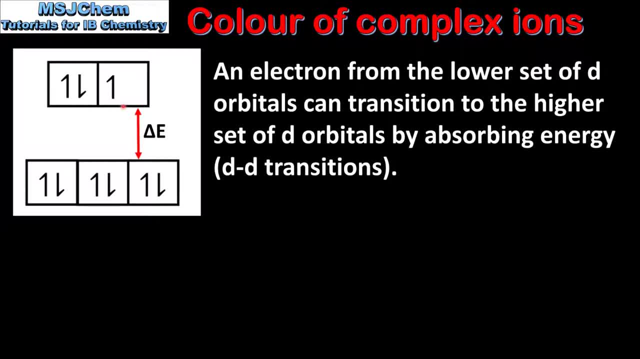 STRANGE EXAMPLE. So in this example, which is the copper 2 ion, we have one 3d orbital which only contains one electron. Because of this half filled d orbital, an electron from the lower set of d orbitals can transition to the higher set of d orbitals by absorbing energy. These are known as d-to-d. 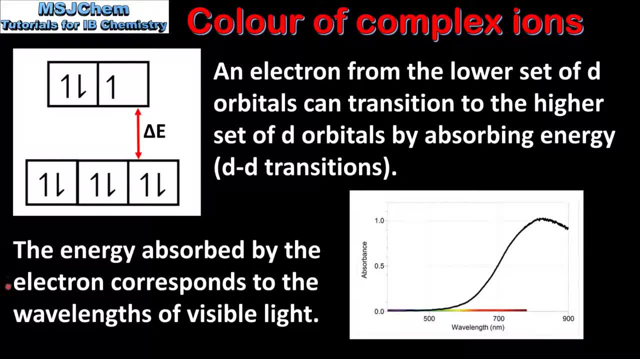 transitions. The energy absorbed by the electron corresponds to the wavelengths of visible light. So earlier we saw this absorption element of the 3d orbital in the bottom of the 3d orbital. So these electrons are now sucked into the energy. And the energy I absorbed in the third orbital is: the same volume. So the energy I absorbed in the third orbital is equal to the distance of the 2d orbital and the distance of the 3d orbitals, As a cross-sections are now separated from the distance of the 3d orbital. 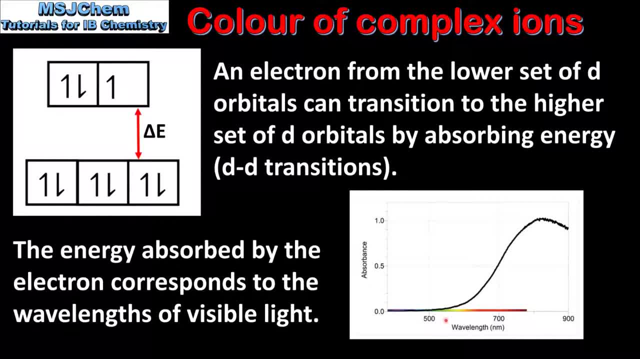 So in this example we see that the 3d orbitals are now separated from the 2d orbital in the first line spectrum for the hexa-aqua-copper-2 ion, And we saw that when white light passes through the solution, certain wavelengths of light are being absorbed and certain 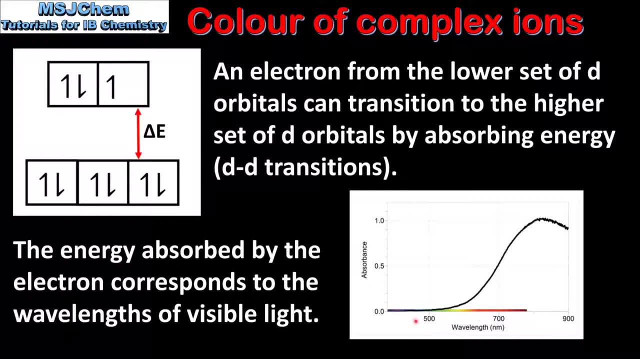 wavelengths are being transmitted. The energy absorbed by the electron when it transitions from the lower set to the higher set of d-orbitals corresponds to the wavelengths of light that were absorbed. The remaining wavelengths of light were transmitted, which we see as blue. So to summarize, the electron. 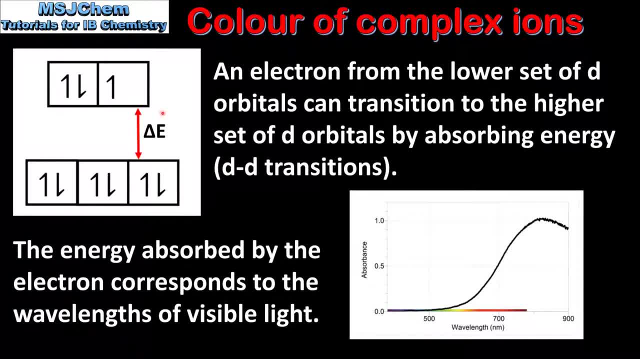 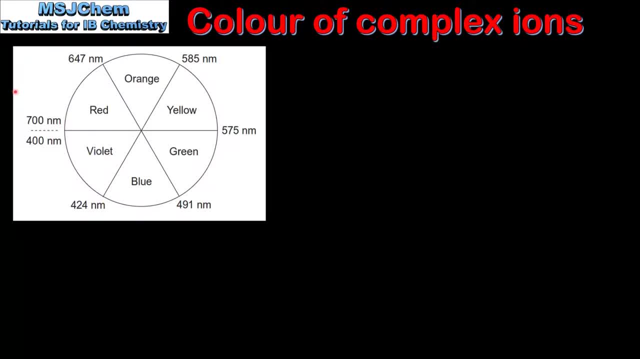 transitions from the lower set to the higher set of d-orbitals absorb energy, which corresponds to the wavelengths of visible light. Next we look at how to use the color wheel to determine the color of a complex ion. The color wheel shows all the wavelengths of visible light, from longer wavelength red light to 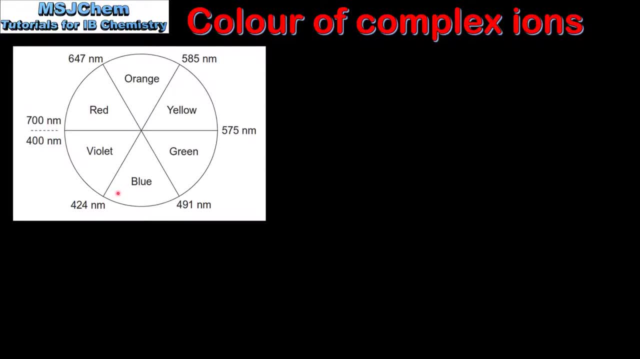 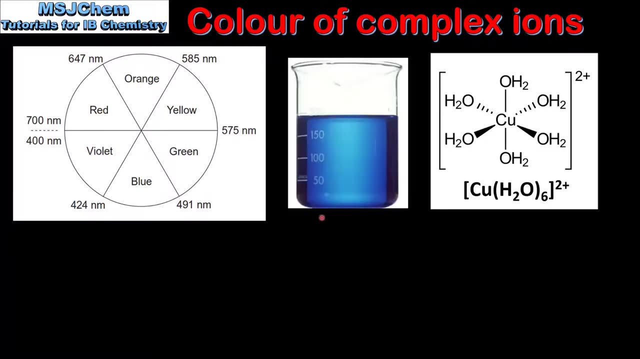 shorter wavelength violet light. The colors that are opposite each other on the color wheel are known as complementary colors. For example, red and green are complementary colors, as are orange and blue and yellow and violet. Earlier we saw that a solution of hexa-aqua-copper-2 ions is 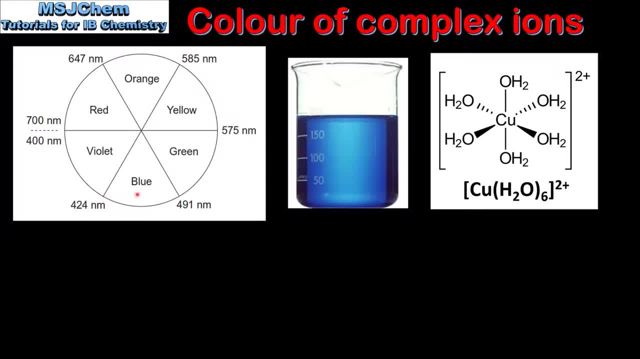 blue. Using the color wheel we can determine which color is transmitted and which color is absorbed. So the hexa-aqua-copper-2 ion appears blue because it absorbs orange and blue. The hexa-aqua-copper-2 ion is orange light and transmits blue light, The color. 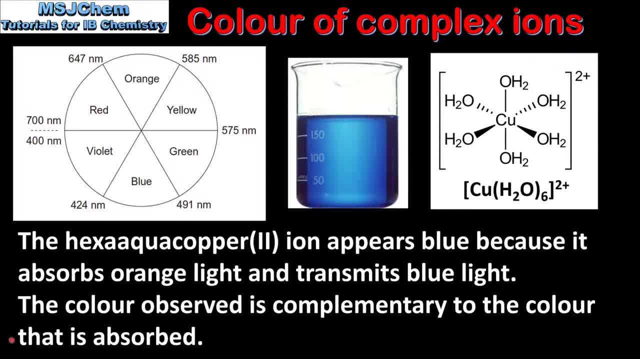 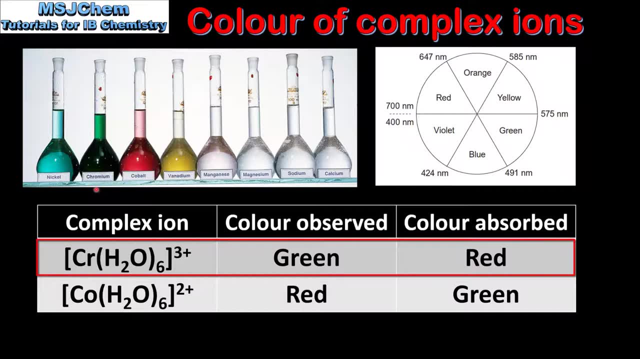 observed is complementary to the color that is absorbed. So for this complex ion, orange light is being absorbed and its complementary color, which is blue, is being transmitted. So next we look at a couple more examples, Starting with this solution of chromium ions, which appears green. So if we use the color wheel, we 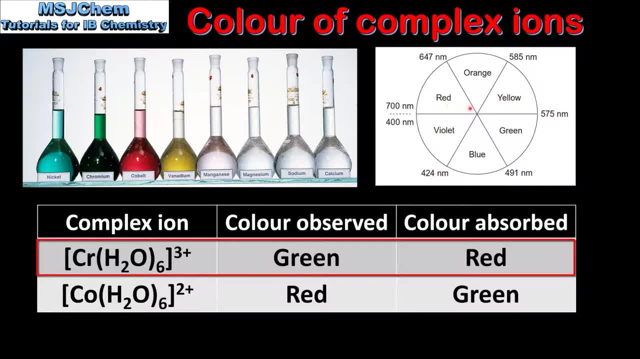 can see that red light is being absorbed and it's complementary color, which is green, is being transmitted. Next we have the solution of cobalt ions, which appears red. So if we use the color wheel, we can see that green light is being absorbed and its complementary color, which is red. 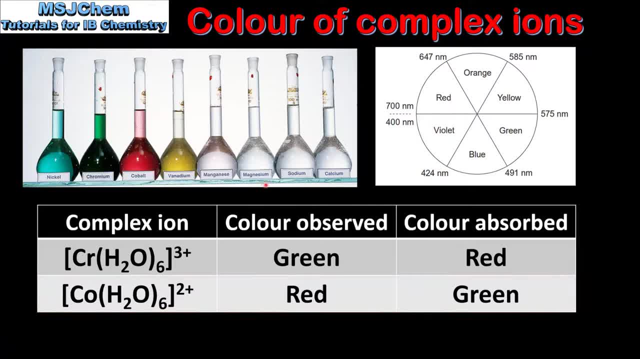 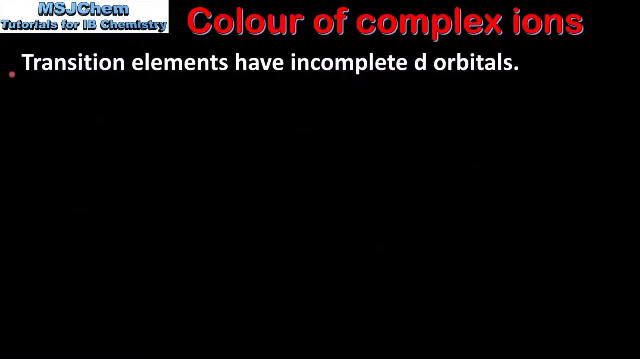 is being transmitted. Note that solutions of magnesium sodium and calcium ions are colorless. This is because they are not absorbing any wavelengths of visible light. So let's end with a summary. As we've seen, transition elements have incomplete d-orbitals. The d-orbitals split into two sets of higher and lower energy when the